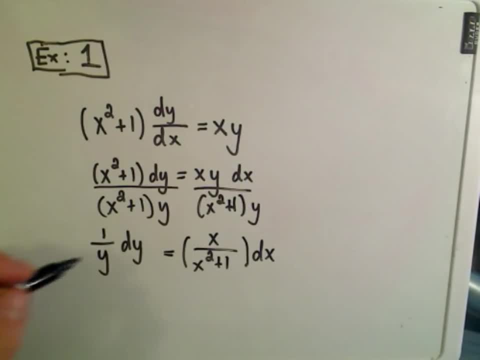 Which is just going to be a function. So that's what we're trying to do here. We're basically trying to integrate and, if possible, solve for y. That'll be our solution. Sometimes it's not always possible to do that, but that's okay. 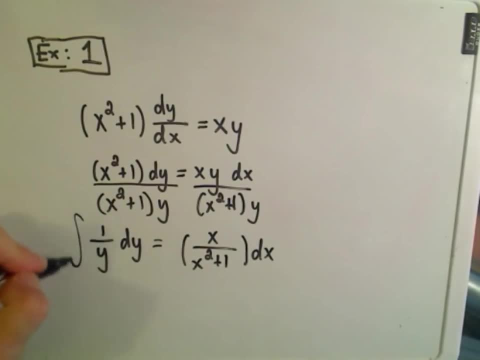 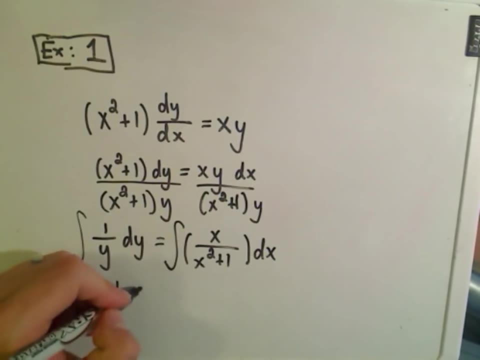 So at this point all we really do is integrate both sides. Well, if you integrate the left side, you get the natural logarithm of y. You know, normally you tag on a plus c. We can just plug it on to one side or the other. 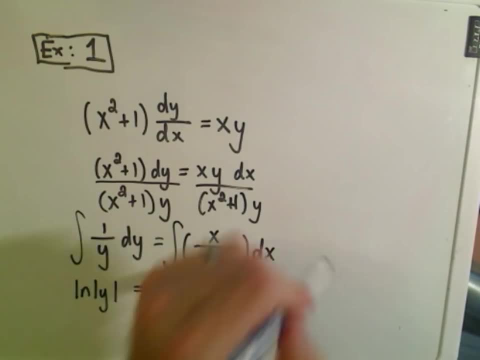 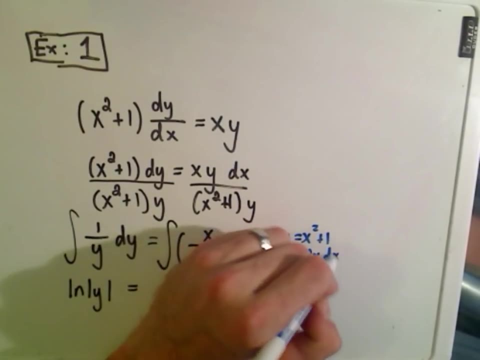 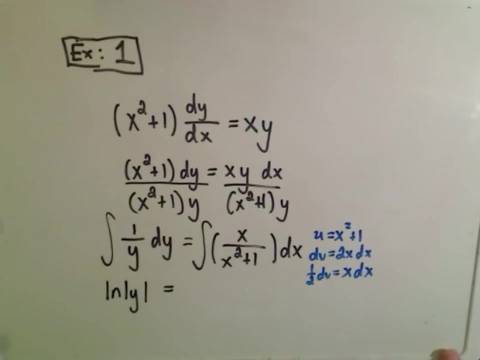 To integrate the right side, I would have to do a u substitution. I would let u equal x squared plus 1. du would be 2x dx. so then I would get one half du equals x dx. So then when I go to integrate it says: really, I'm going to be integrating. well, xdx is replaced by the. 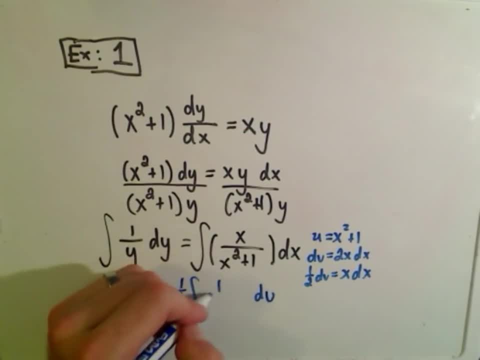 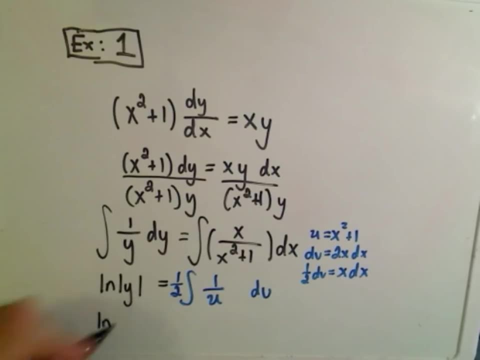 one-half du, and then I'm just going to have 1 over u left over. So when I integrate both sides again, on the left I already have the natural logarithm of y. I'm done with that. On the right, I'll get one half the natural logarithm of u, but remember u is x squared plus 1. 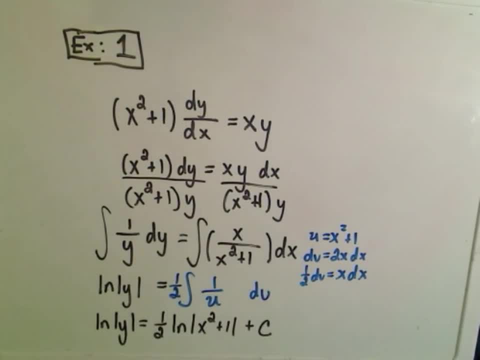 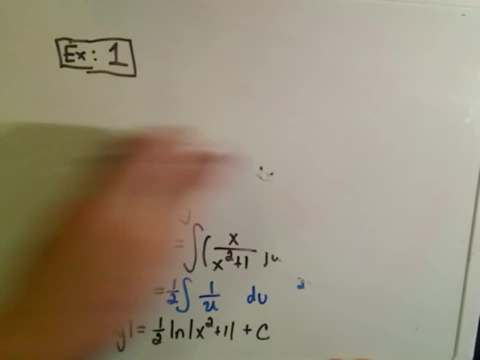 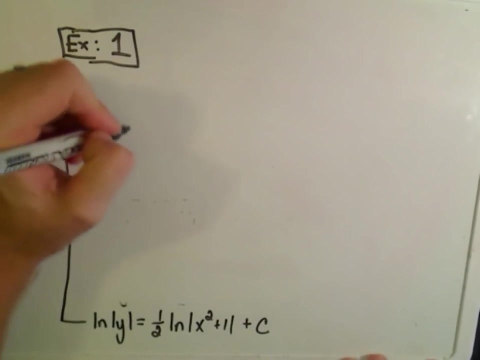 plus 1. plus c Now, if possible. usually what you'll do on these is try to again get it in terms of y. Okay, so I'm going to get this in terms of y here real quick, and remember to get something to get rid of natural logarithms. you. 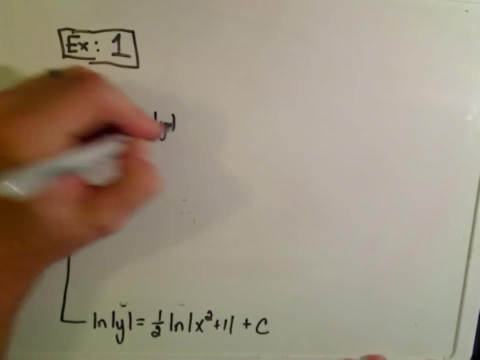 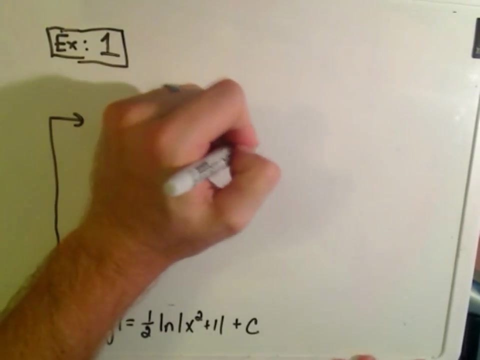 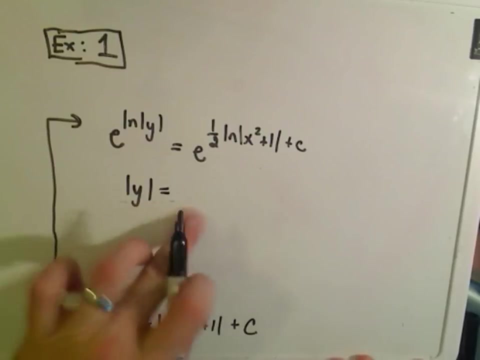 exponentiate both sides. So I'm going to take e raised to the natural logarithm of y, and then I'm going to take e raised to the one-half natural logarithm of x squared plus 1. plus c, So we'll be left with absolute value of y equals. 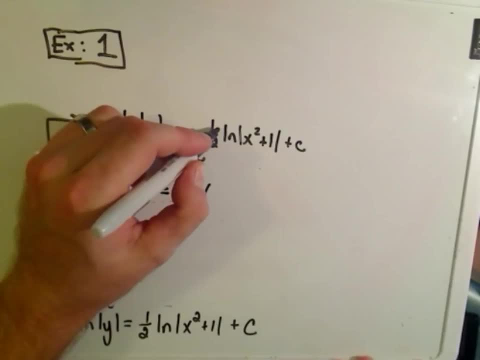 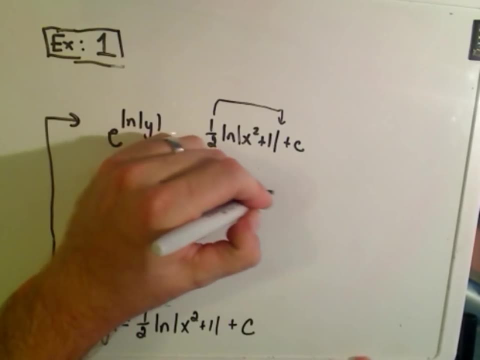 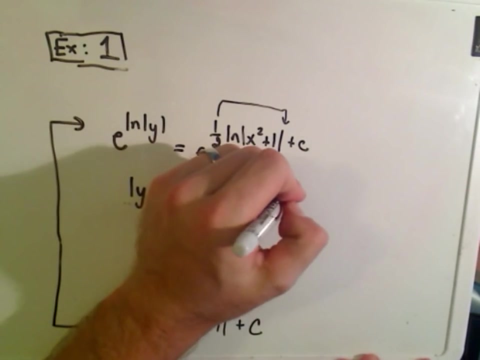 Remember the other trick too: You can bring coefficients up as exponents on logarithms. So really I'll have the logarithm, but the exponent of one-half will turn into a square root, So I'll have the natural logarithm of x squared plus 1.. 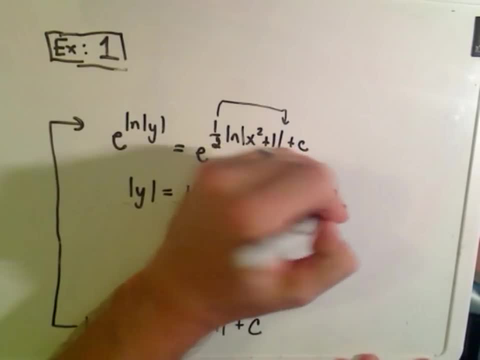 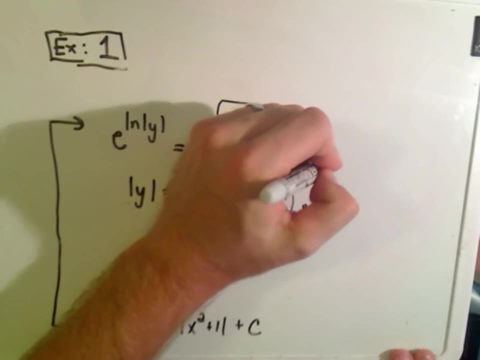 I could write this: times e raised to the c. Okay, so I could have written it as e to the part times the e to the c. right, I could have written this as e to the one-half. the natural logarithm of x squared.